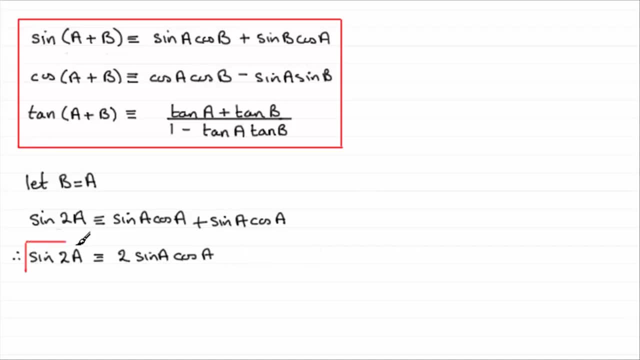 Now, if you forget these identities, you can always build them up from these results. So it is your understanding that really matters here. Okay, well, I'm not going to do the cos one at the moment, because that's a bit more involved. 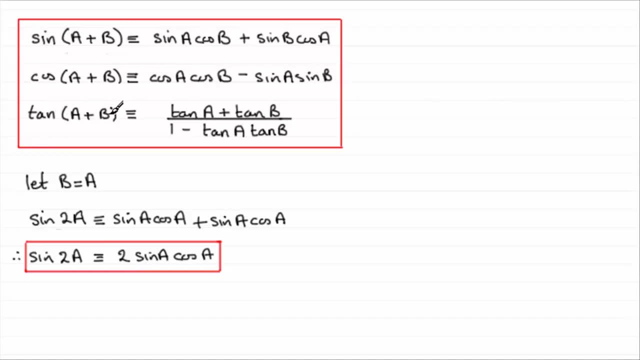 But you might like to try this one, The tan of a plus b. we know is tan a plus tan b all over 1 minus a. So we're going to do the tan of a plus b all over 1 minus a. So we're. 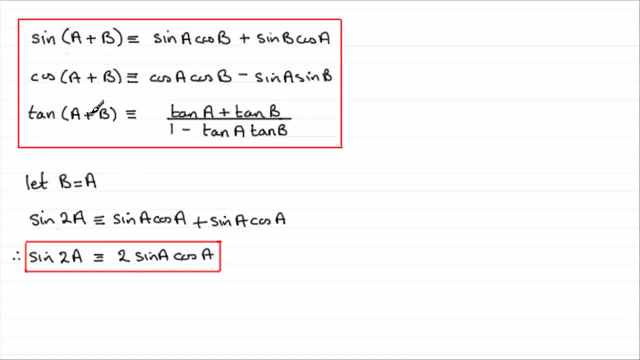 going to have tan a plus tan b. By doing a similar thing like this, you should be able to work out what the tan of 2a is, So maybe you might like to just give that a try. Okay, so let's see what we get. So if we replace the b with an a, we're going to have tan of. 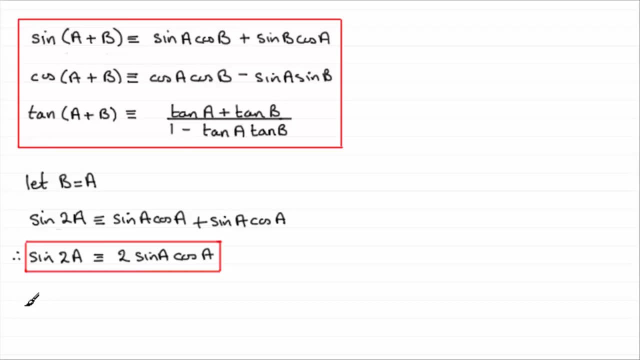 a plus a, which is the tan of 2a. So tan of 2a is identical to tan of a plus a. So tan of 2b is equal to tan a plus another tan a. So in other words we have two lots of tan a on the top. 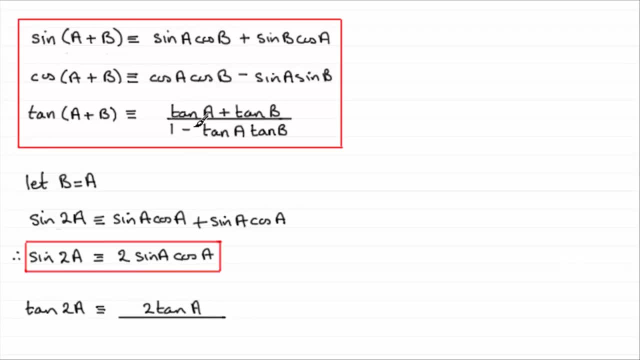 And then all of this is divided by 1 minus tan a times another tan, a Tan squared a, in other words. So on the bottom here we have 1 minus tan squared a. So it would be good if you got that one. Okay, let's just highlight this Now. I said I was going 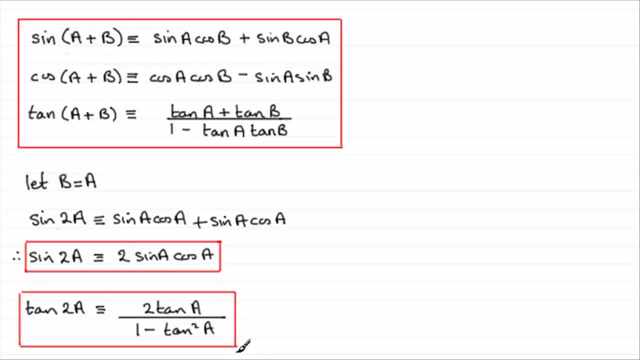 to leave the cosine one to the end, because it's a bit more involved. So you might like to again have a go at coming up with an identity or two, And that's a little hint. There are several identities that you can get for the. 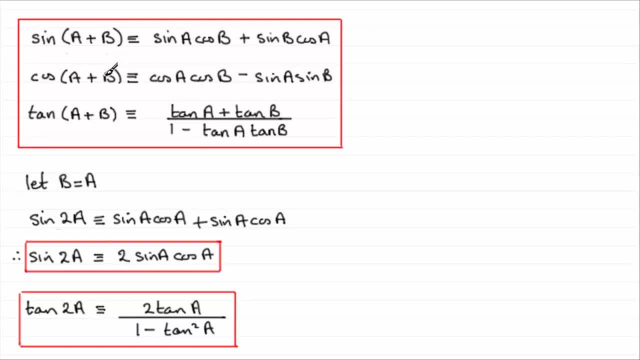 cosine of 2a. Have a go see what you come up with. Okay. well, let's see. how did you get on? Well, let's start with cos 2a then, where we replace the b with an, a. Cos 2a is going to be identical then to cos a times another cos a. 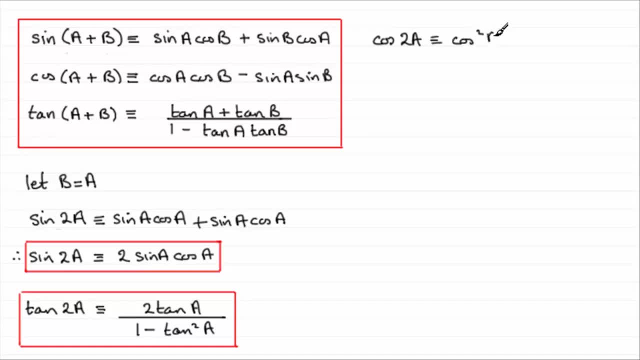 cos 2a, in other words Minus, and we've got sin a times, another sin, a sin 2a. So did you get that identity? Well, if you did, well done. But what we can do is we can go on. 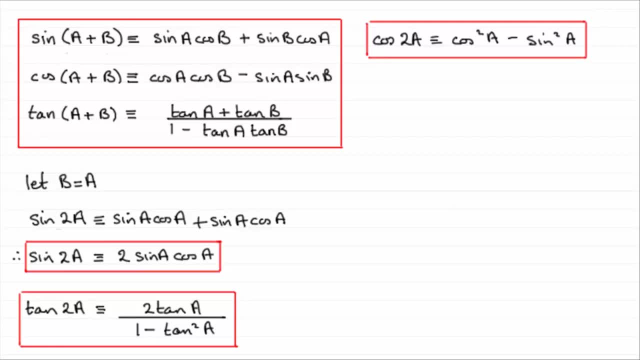 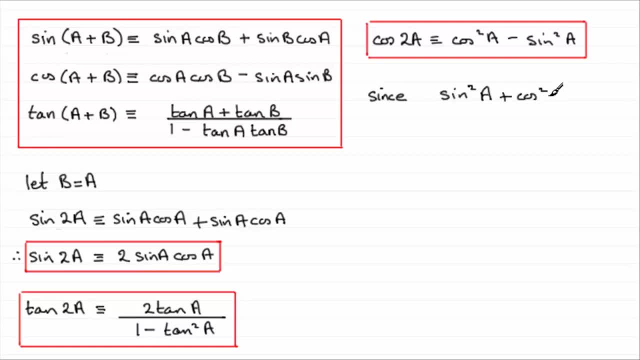 let's call it a plus cos 2 of any angle, or cos 2 plus sin 2 of the same angle, doesn't matter which way round we have, this always comes to 1.. We can use this identity to change this result up here, Because, for instance, sin 2 a. 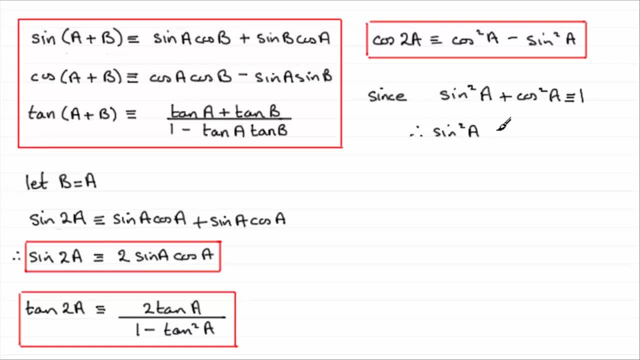 let's just write it in: if we were to rearrange this, sin 2 a would be identical to 1 minus cos 2 a. And also if we made cos 2 a the subject, we'll just say also cos 2 a would be identical to 1 minus sin 2 a. So what we can do is we could put this result: 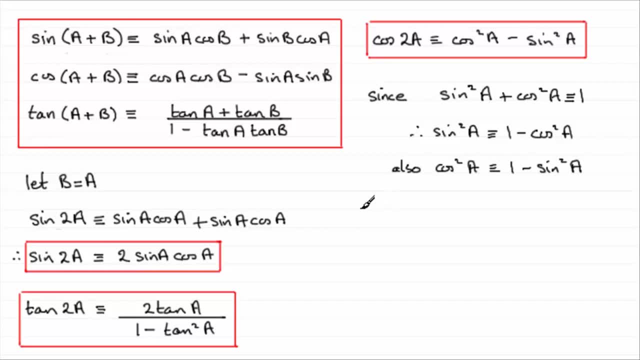 into our identity up here. So what we end up with is if we replace the sin 2, a with 1 minus cos 2 a in here you've got to be very careful with this one. Cos 2 a would be identical to the cos 2 a here, and then we've got minus and then replacing 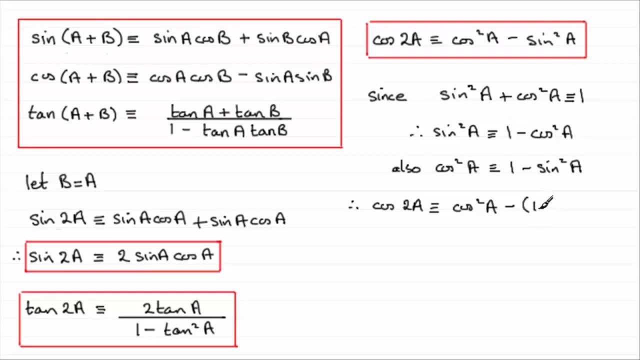 sin 2 a with 1 minus cos 2 a. There's a couple of terms here, so you've got to be careful. You've got to put that in a bracket. So if we open up this bracket, if we expand it, 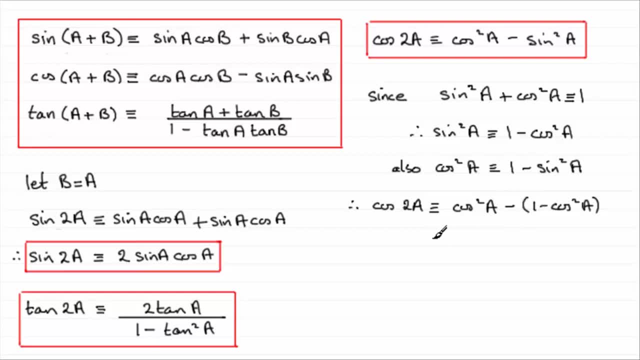 multiply it out with a minus 1. that's here what we end up with. we've got to be careful. we've got to be careful, we've got to put that in a bracket. So if we open up this bracket, 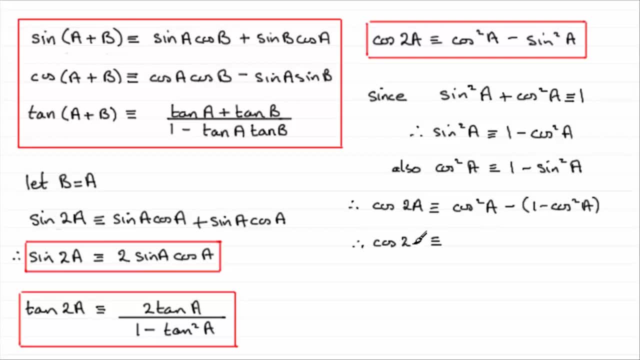 with is that, therefore, cos2a turns out to be cos2a, and we've got minus minus here, cos2a making another plus cos2a. So we end up with cos2a plus cos2a, which is 2cos2a, And then